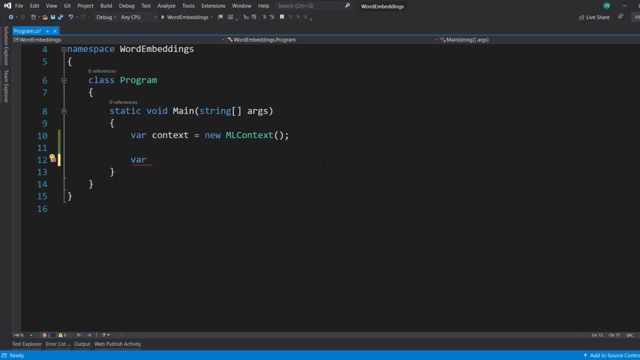 And using word embeddings within MLNET it's going to use a pre-trained word embedding And so we don't need to give it any data. We can just pass in some empty data And we can do contextdata, load from it enumerable, And I'm going to load in a new list text input: 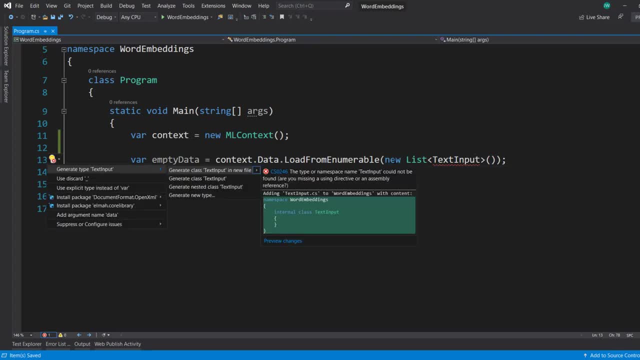 And let's go ahead and create this input class here. It's just going to have a property string and it's going to be called text. So we have our empty data. Now let's create our embedding pipeline And the first thing we need to do in the transforms at text is to normalize our text And we give 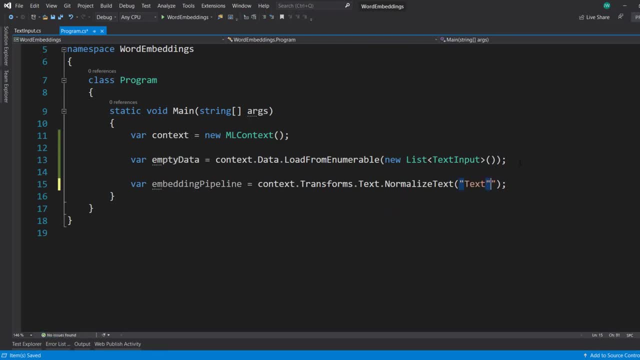 it the output column of text And since we don't have any input columns that we need to give it, I'll just say no for our input column name. And if you recall from our normalized text video, there's a few properties that we can do. I can say keep diacritics And then 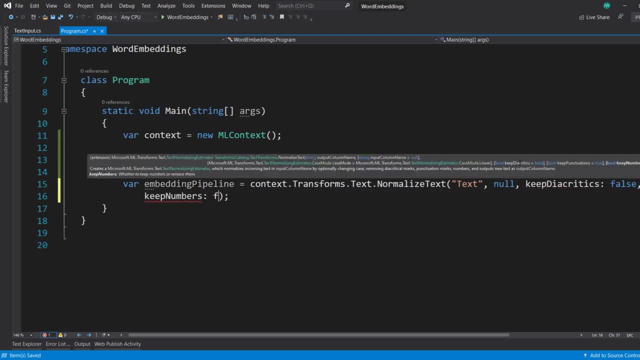 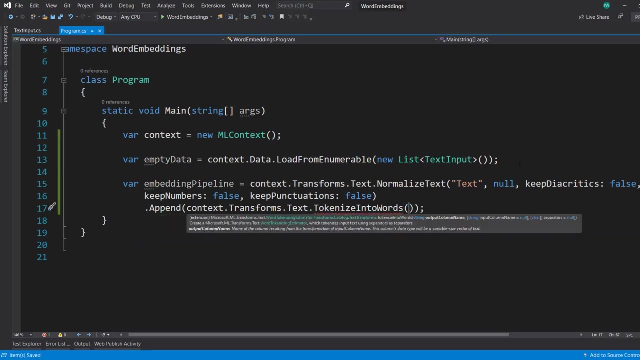 I can say: keep numbers as false. I'll say: keep numbers as false as well as keep punctuations as false. Next I'm going to append another transform and that's going to be tokenized into words. So we normalize our text first And then we tokenize that text into a single words there. 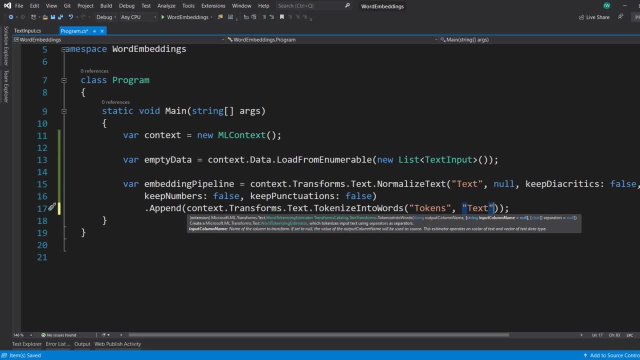 Output column into tokens. Input column into text, because we call this output column as text, So we're just going to use that and I do another append. This time it's going to be context that transforms text. This is where apply word embedding Output column. I'll do features. Input column is going to be tokens. 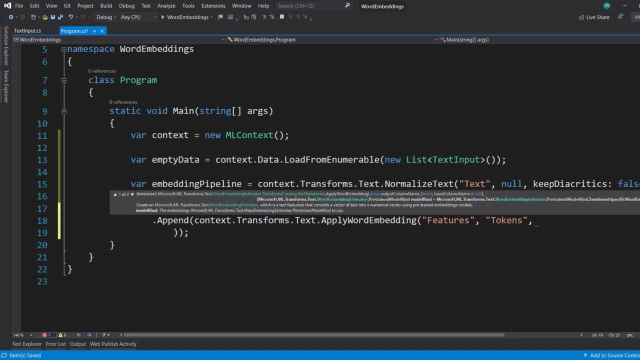 And our third parameter here is the model kind. This is where we tell what kind of pre-trained model that we want to use within our word embeddings. You see it comes in with quite a few. Glove is the most common one here And the number with the D that tells you. 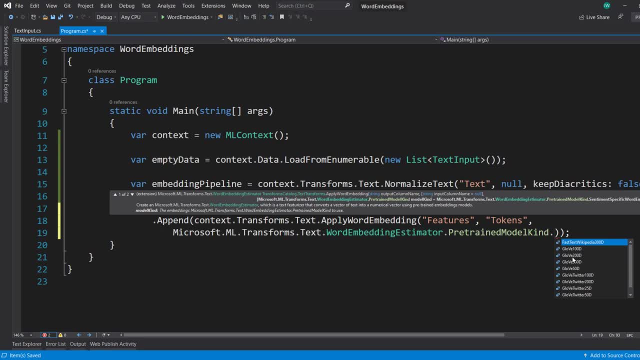 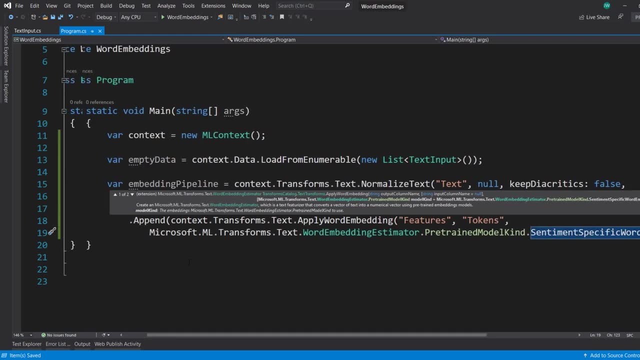 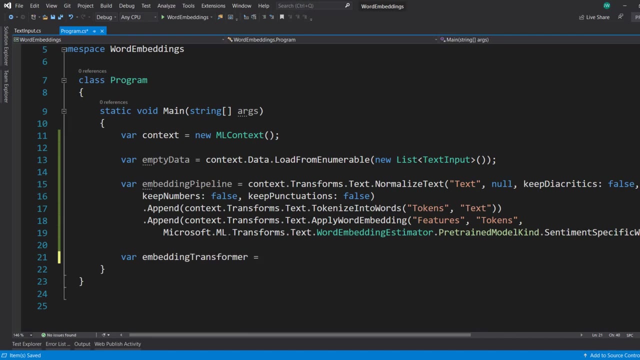 how many dimensions it has been trained on. So the higher the number, the higher dimensions the model has been trained on. I'll just use the sentiment-specific word embedding here And we'll get our embedding transformer. We're calling our pipeline that fits on our empty. 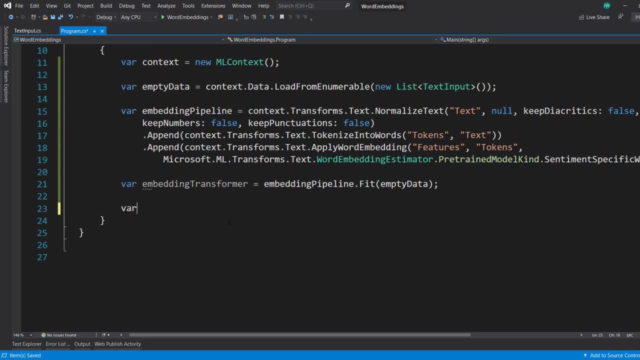 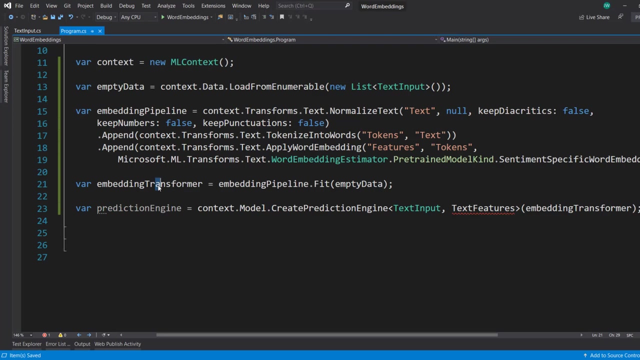 data. Okay, Next I'll create a prediction engine with context model. Create prediction engine, Use that text input And I need to create a text features output schema. But I'll go ahead and pass in the embedding transformer or the model that we got from our pipeline. 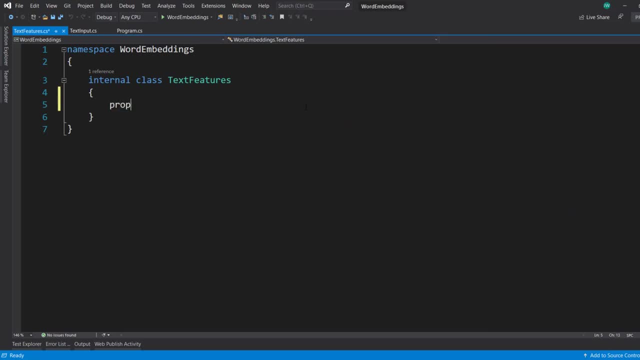 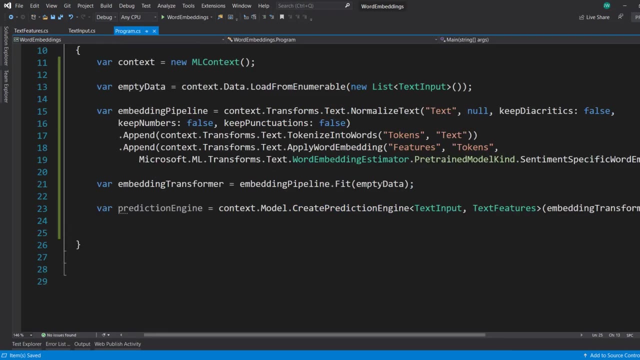 So I'll create this file And that's just going to have a single property, a float array, And it's going to be called features. So we have our prediction engine. Let's predict on a couple of things here. First, let's do a new text input. We give it a text of. let's 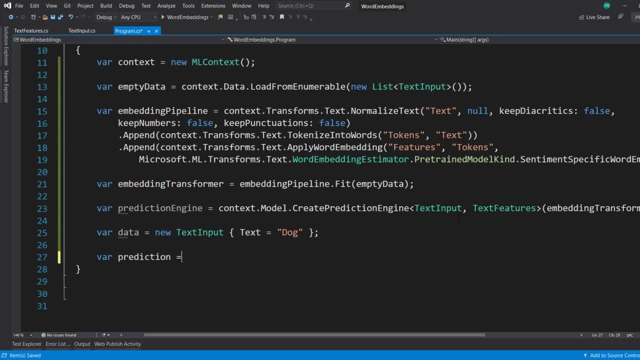 say dog, And we get the prediction from it using the prediction engine to predict on that new data, And what we can do is write out to the console. Okay, First we do the number of features And that's going to be the prediction that features. 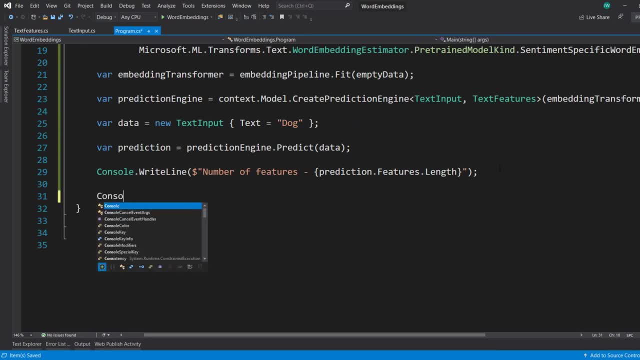 that length And next we'll print out the actual features, which is going to be the vector of the embedding for that single word. To do that, we do a for each, So for each feature and prediction that features, Remember, these are: 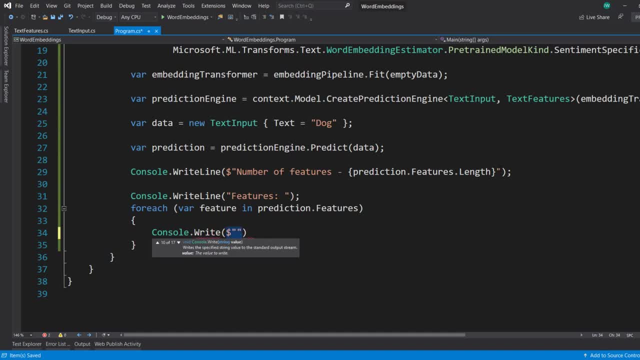 Floats. So we're going to get numbers here, The consolewrite, And I do Just do feature, Add a space there And you know what? Let's do another one. So I do a consolewrite line environment, that new line, to kind of space it out, make it easier to read our output here.